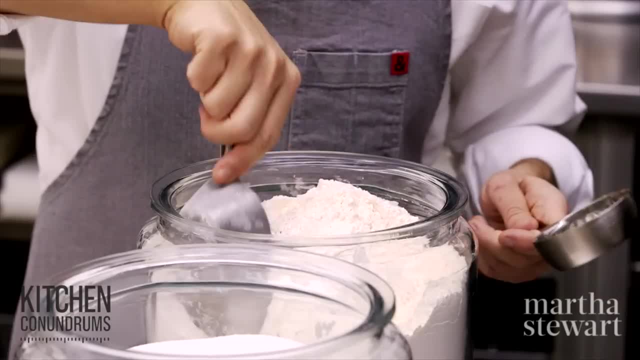 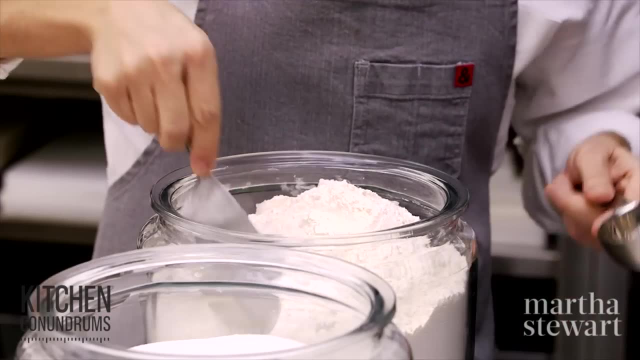 lightening it, incorporating a little bit of air, because as this canister of flour sits on your shelf, it actually compacts itself, It settles on itself. So give it a little bit of a fluff here and scoop it into your cup, sprinkling it in using that offset spatula, anything with a straight side. 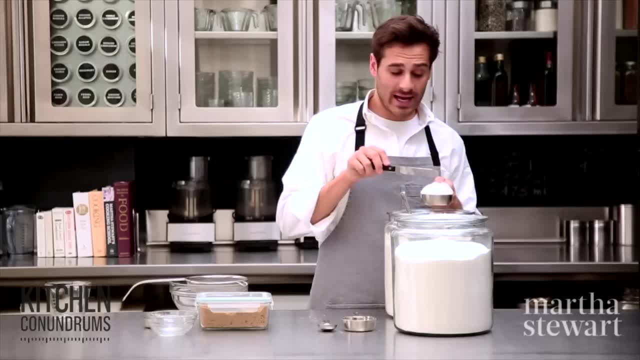 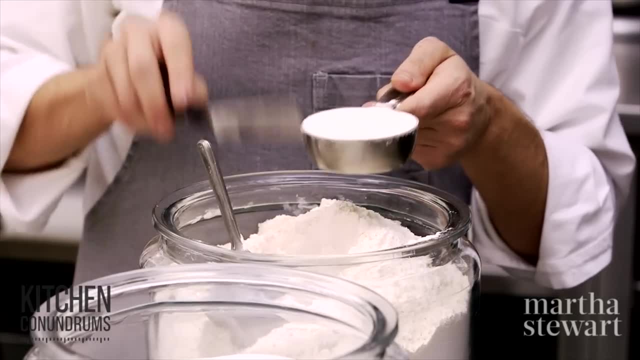 You want to give the cup a little bit of a tap, settling in any air pockets that might be in this cup of flour and a good swipe leveling it off, And that is a perfect half cup of flour. Now, if a recipe calls for sifted, 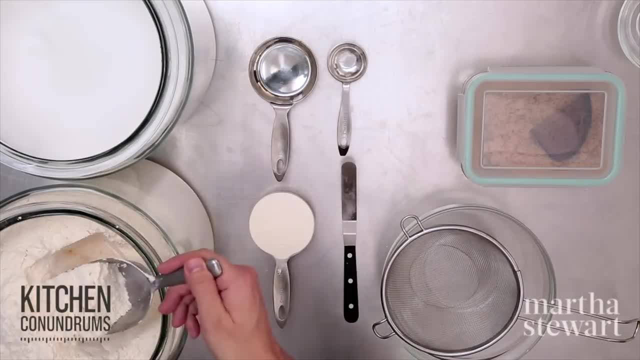 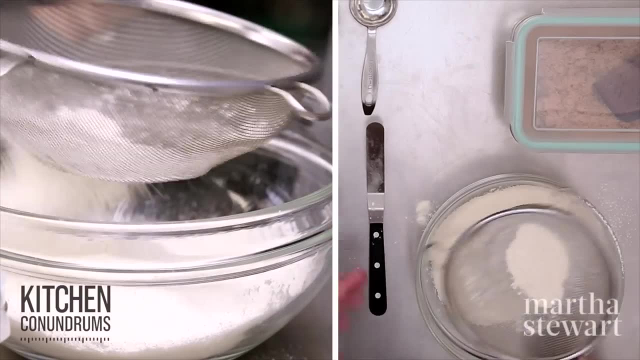 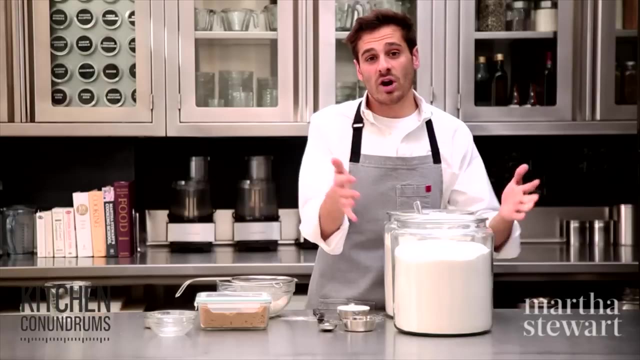 flour. what that means is that you need to sift the flour first and then measure from this bowl. measure this mixture here, And what that means is you're getting a lighter cup of flour, something that isn't so heavy. Okay, Now, something like sugar. sugar is already dense, so there's no need to stir it up and you don't need. 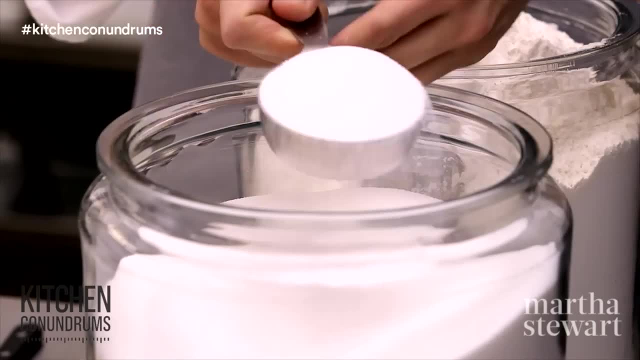 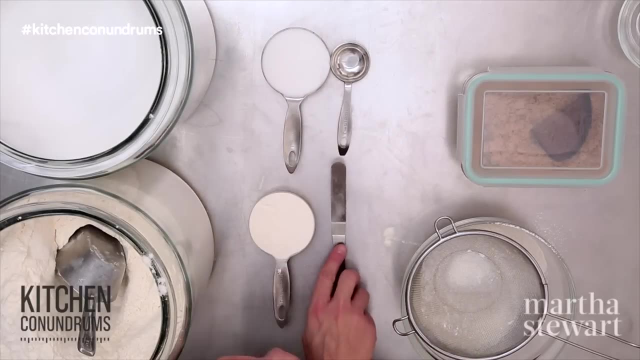 to scoop into the cup. You can simply dip your cup into the canister itself and give it a good swipe, And the weights would be completely consistent here. This is a perfect half cup of sugar. Now brown sugar. We get a lot of questions here in the test kitchens: How do I keep my sugar from getting 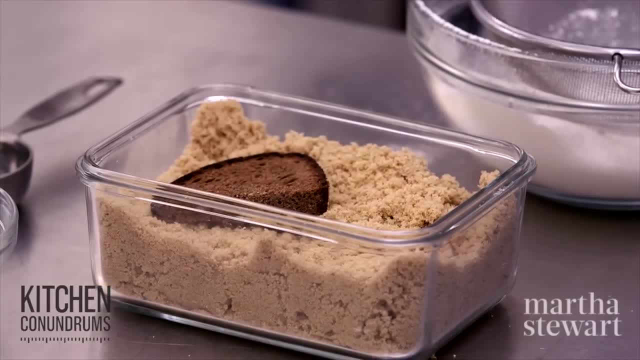 too hard. Keep it in a well-sealed container. One of these airtight containers is really great. Take a piece of bread. Some people like to use a little bit of sugar. Some people like to use a little bit of flour. 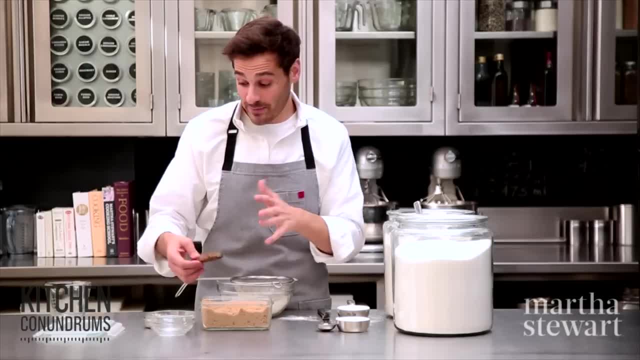 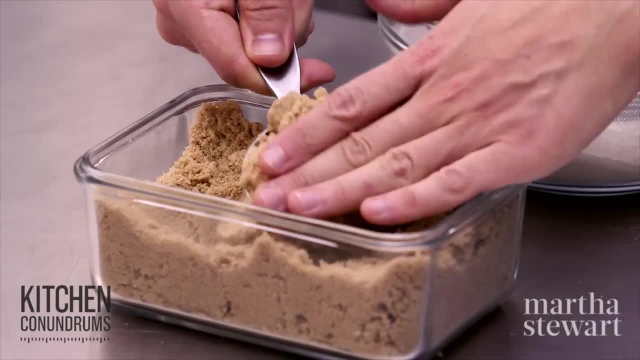 Some people like to use a piece of apple and store it in with your brown sugar, and it will help to keep the sugar nice and soft. Take your measuring cup, dip it into the brown sugar and pack the sugar into the cup. Most recipes call for packed brown sugar. 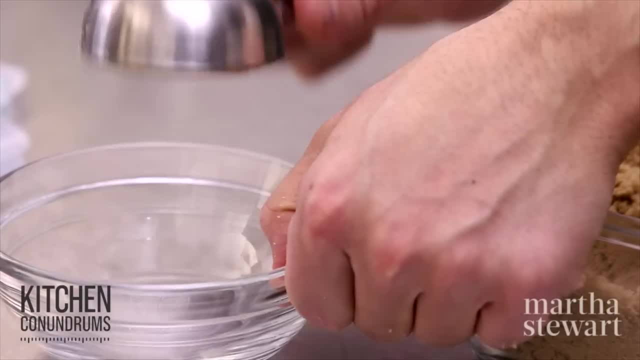 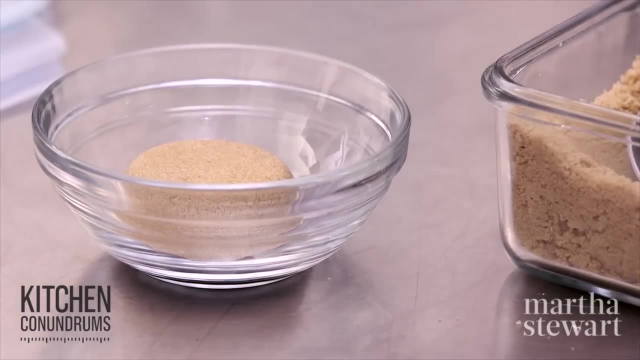 Now you know you've done this right. if you tap it out into a bowl and the sugar holds its shape, If it crumbles, that means that you haven't packed it firmly enough and that you should start over. So now for liquid measurements. Use a spouted glass bowl.